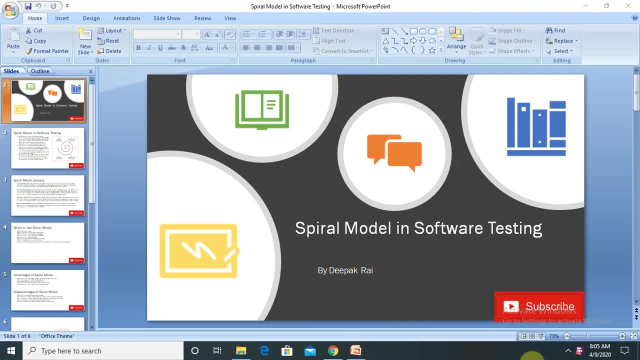 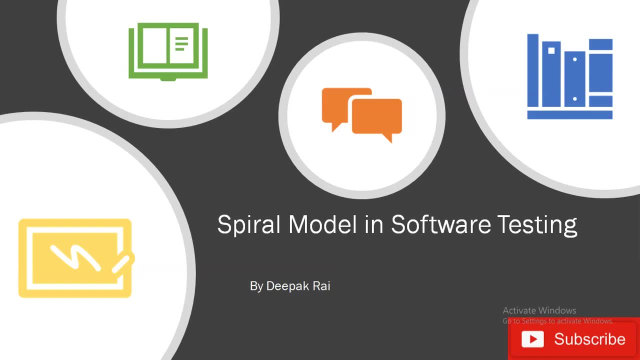 Hi everyone. welcome back to our new session of the software testing. So in this session we will learn about spiral model in software testing. As I said in my previous session, V model, spiral model and waterfall model is basically an important part in the software development life cycle, But testing is also a major part covered in development phases. 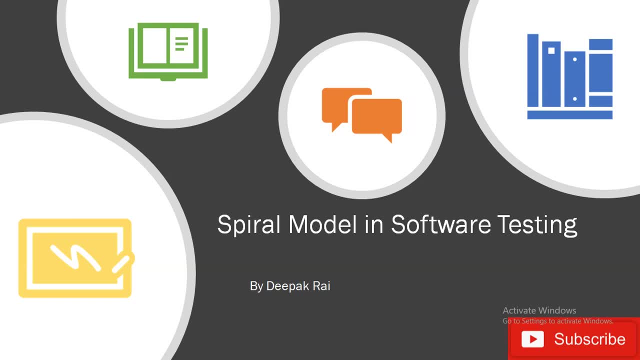 So we have to learn these models in software testing as well. For complete understanding, please be available from start to end of this tutorial And for those who are looking for this PPT, please drop your email ID in comment section. I will forward your email ID. 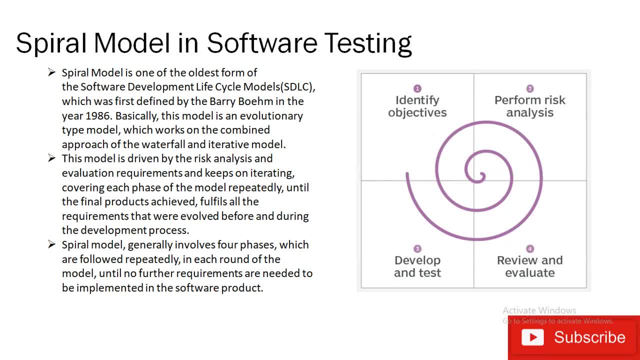 So let's begin with this. So first of all, what is spiral model in software testing? So spiral model is one of the oldest form of software development life cycle models, which was first defined by Barry Bohem in the year 1986.. Basically, this model is an evolutionary type model which works on the combined approach of the waterfall and iterative model. 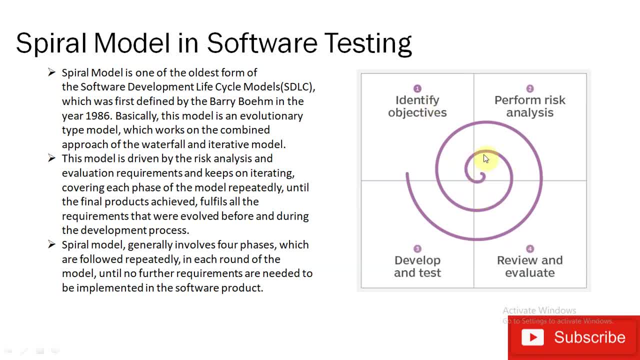 So, as you can see here, the diagram itself is a spiral, So you can see its spiral. because of that, its name as suggested spiral model. So you can see four major phases are include 1,, 2, 3, and 4.. So identify objectives, perform risk analysis, develop and test and re-evaluate. 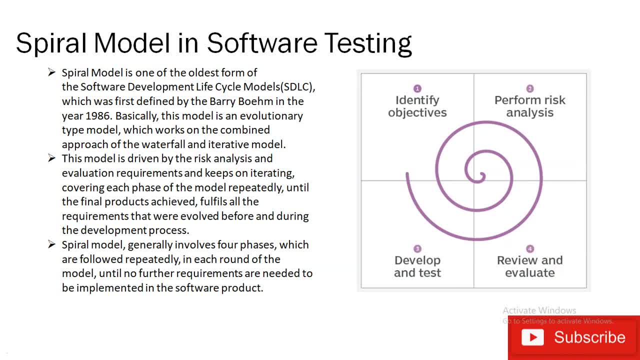 The popular spiral model is a blend of both iterative development method as well as sequential improvement model. That is the waterfall model That is having exceptionally high importance on risk analysis. In this model, the exact number of phases for developing a product varied based on some constraints and by project manager, which calculates the project dynamics, project risk. 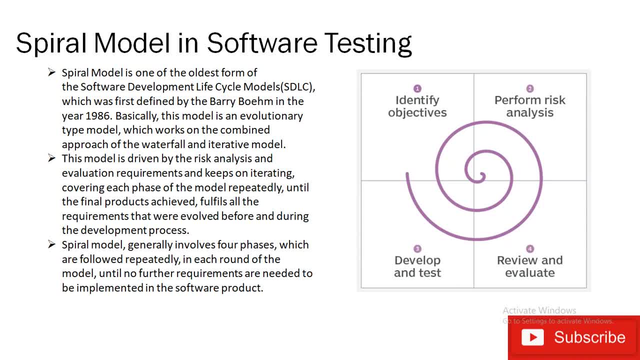 Here the project manager dynamically resize the number of phases and hence play a significant role in the development of a product using the spiral model. The radius in spiral model usually shows the expenses or cost needed for project development. Angular dimension shows the development done today during the recent phases. 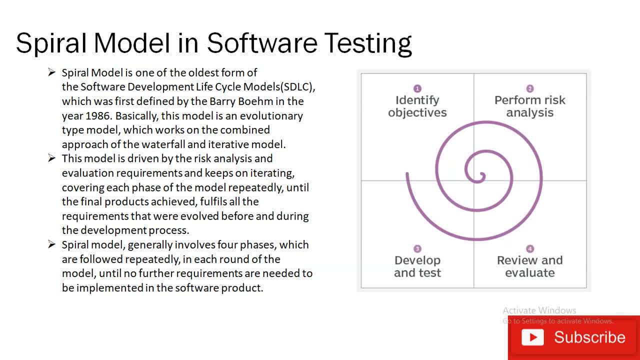 So this model is driven by the risk analysis and evolution requirements and keeping on iterating, covering each phase of the model repeatedly until the final products achieved Fulfils all the requirements that were involved or evolved before and after. Spiral model generally involves four phases, as I have already explained here. 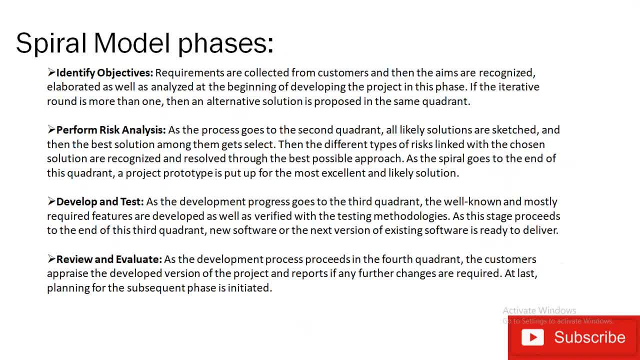 So let's jump to the next point. So we can see here in the previous diagram, the spiral model looks like a coil with many loops. The number of loops varies based on each project and is often designed by the project manager. Each loop of the spiral is a phase in the software development process. 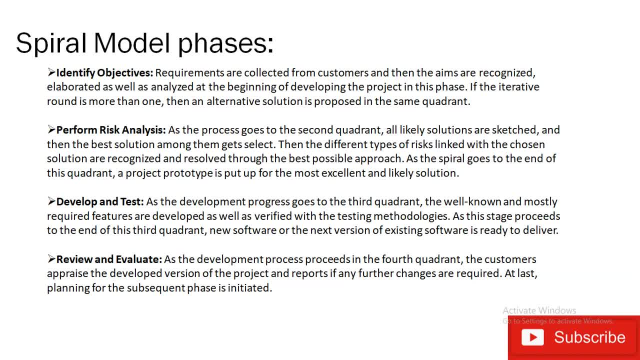 The spiral model enables gradual release and refinement of a product Though each phase of the spiral, well as the ability of build prototypes at each phase. The most important feature of the model is its ability to manage unknown risk after the project has commenced or announced. 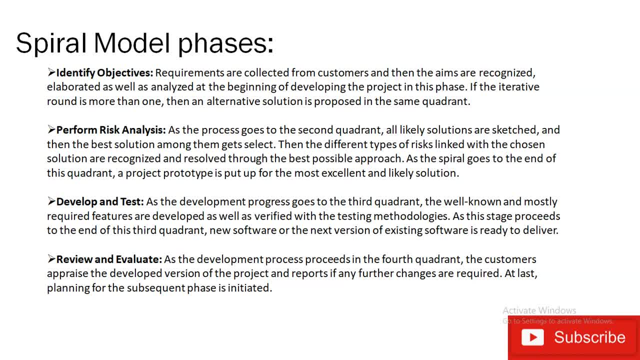 Creating a prototype Makes this feasible. So there are different phases. We will discuss each and everything. So identify objective is the first phase. Requirements are gathered during the planning phase. in this phase, Requirement like BRS, BRD document, or you can say business requirement specification or business requirement documents. 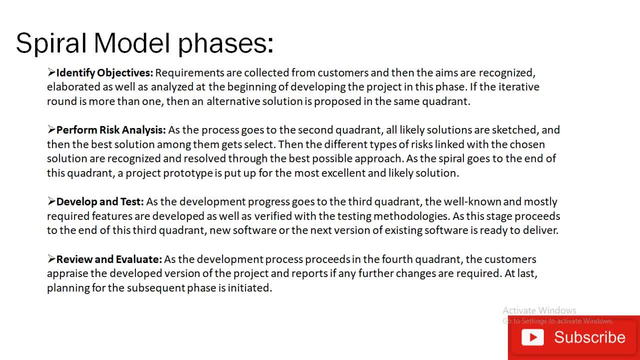 That is, system requirement specification also required. So requirements are collected From customers or end user or the owner, And then the aims are recognized, elaborated as well as analyzed at the beginning of developing the project. in this phase, If the iterative round is more than one, then an alternative solution is proposed in the same quadrant. 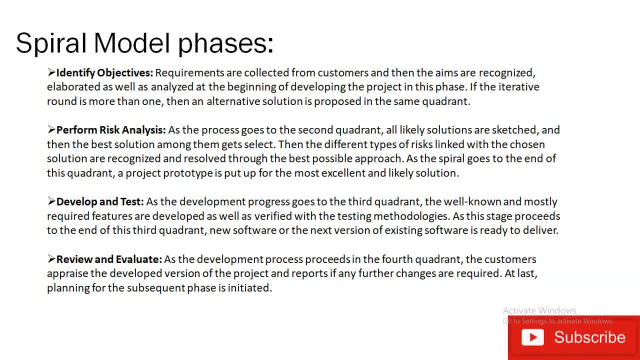 Next is perform risk analysis. So, as the process goes- the second quadrant- all likely solutions are sketched And then the best solution among them gets select. Then the different type of risk linked with the chosen solutions are recognized and resolved, Though the best possible approach as the spiral goes to the end of this quadrant. 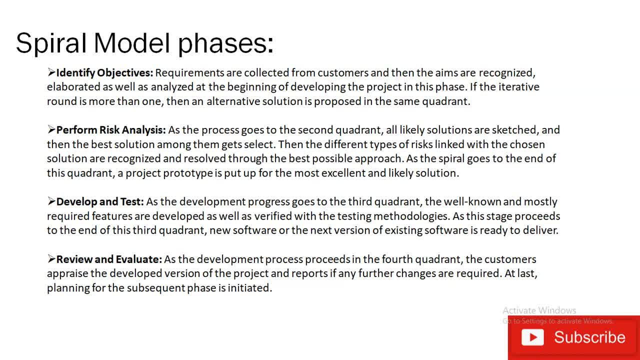 A project prototype is put up, the most excellent and likely solutions. Third is develop and test. So before that, if you want to include some more point on the risk analysis. So risk analysis phase is the process of undertaking to identify risk and alternate solution. 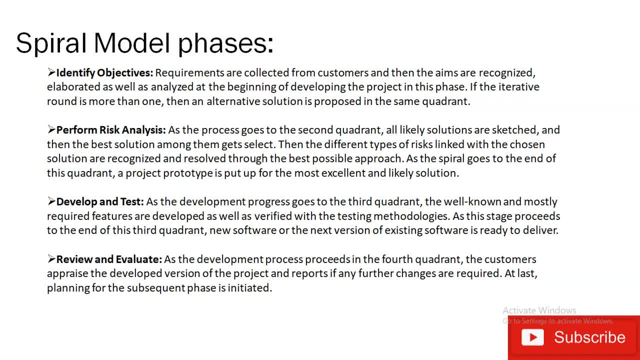 A prototype is produced at the end of the risk analysis phase. If any risk is found during this risk analysis, the alternate solution is suggested and implemented. So next is develop and test. So in this phase is also called as development phase. So development progress goes with third quadrant. 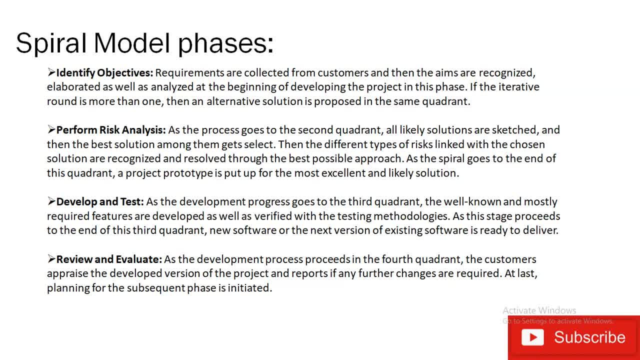 The well-known and mostly required features are developed as well as verified. So within this phase testing methodologies also introduced. As this stage proceeds to the end of third quadrant, new software or the next version of the existing software is already delivered. So in this phase software is developed along with testing at the end of the phase. 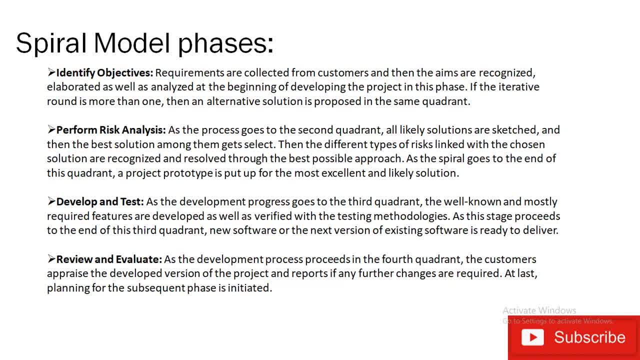 Hence this phase is development, and testing is done here Now review and evaluate. So as the development process proceeds. in the fourth quadrant, the customer appraise the developed version of the project and reports if any further changes are required. At last, planning of the subsequent phase is initiated. 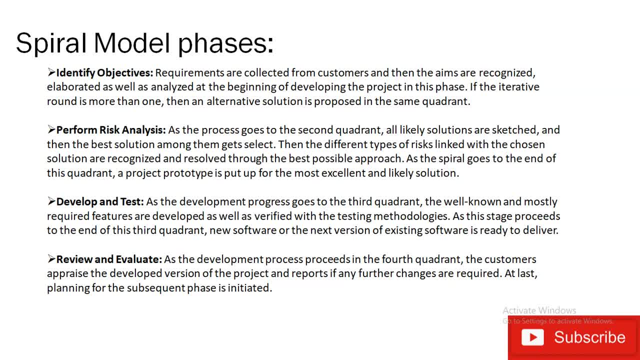 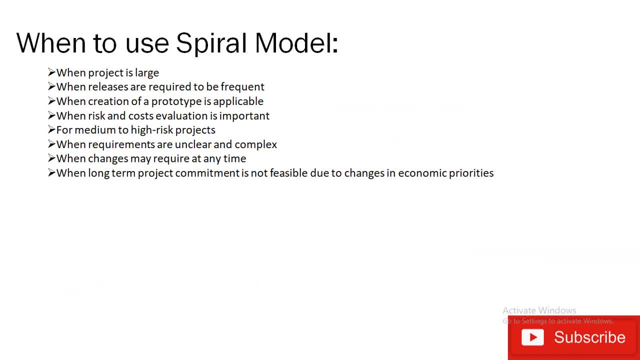 This phase allows the development of the project. This phase allows the customer to evaluate the output of the project to date before the project continues to the next spiral. So when to use spiral model is a major concern. when we are using spiral model, So when project size is very big, like flipkart type of a website or any other e-commerce site or Amazon website. 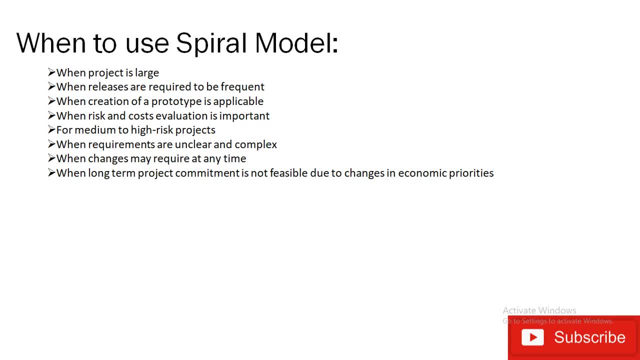 So these type of project will always required spiral model When release are required to be frequent. So just like if we are talking about the development is done in a small, small pieces, be it or chunk in pieces. So that time spiral model is a very useful 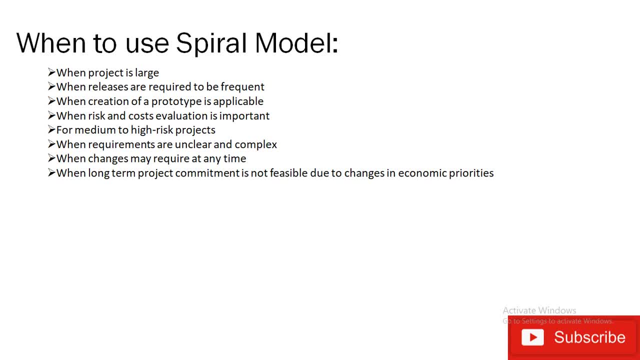 When creation of prototype is applicable or when risk and cost evaluation is important For medium to high risk. project is also introduced for spiral model When requirements are unclear and complex, Just like if you are talking about the any example, like end user wants to develop any application but the requirements is not clear. 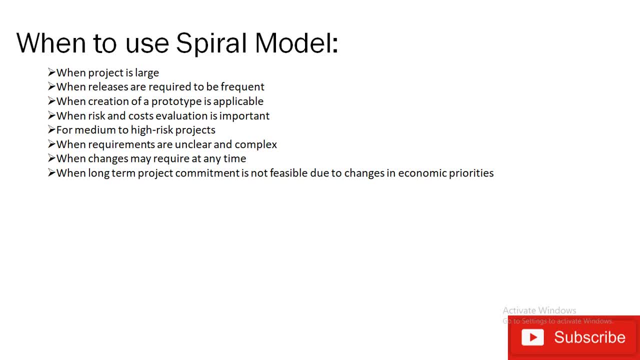 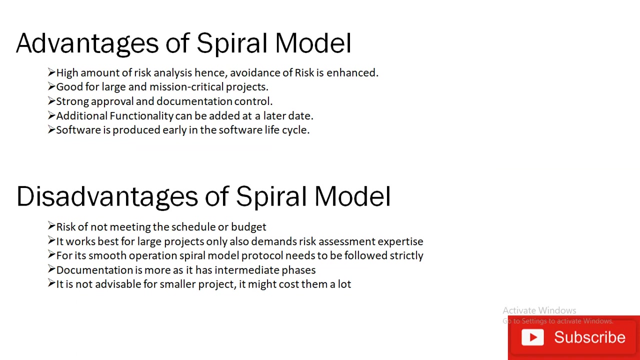 Which all functionality they want to include on that application that time. also, spiral model is very helpful When changes may require at any time and at the end when long term project commitment is not feasible Due to changes in economic priorities. Let's begin with advantages and disadvantages. 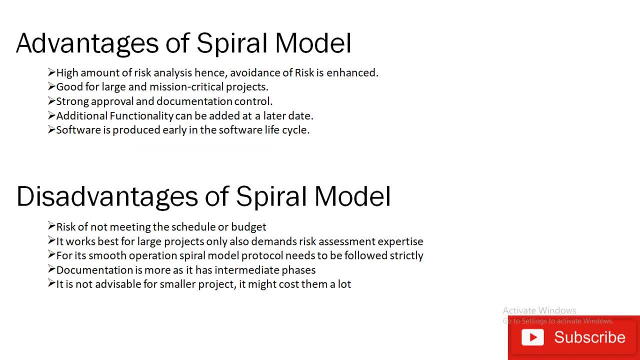 High amount of risk analysis, hence avoidance of risk, is enhanced. Good for large and medium critical project. Strong approval and documentation control. Additional functionality can be added at a later date. Software is produced early in the software life cycle. Then what is disadvantage of spiral model? 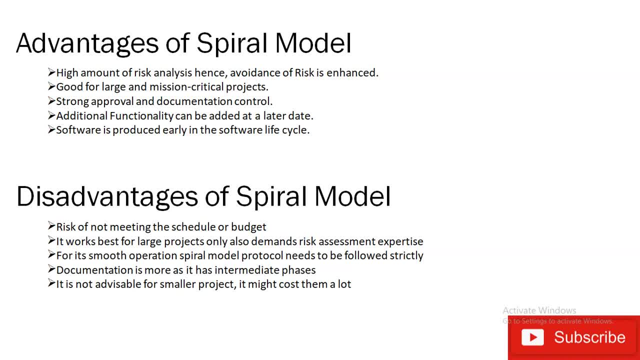 Risk of not meeting the schedule or budget. It works best for large projects only also demands risk assessment expertise. For its smooth operation, spiral model protocol needs to be followed strictly. Documentation is more. as it has intermediate phases, It is not advisable for smaller project. 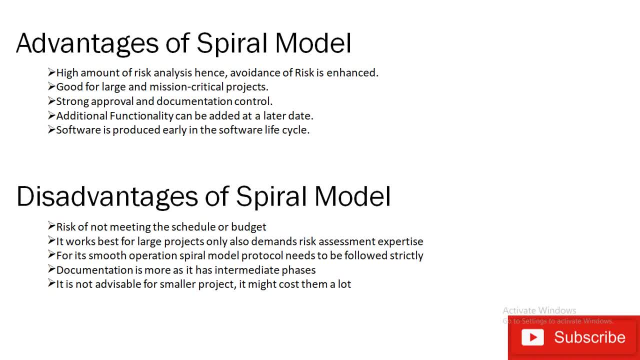 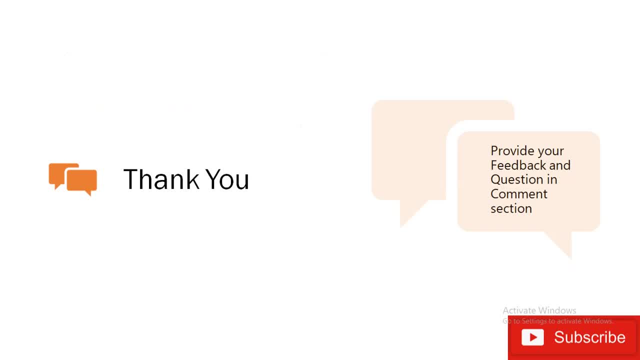 It might cost them a lot. This is all about the advantages and disadvantages of spiral model. Now here everything is complete on spiral model. Hope you understand it. If you have any queries or comment, please comment in the comment box So that I will check and reword the resolution.